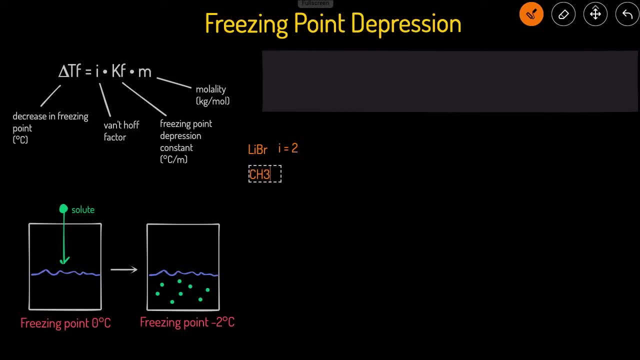 up. But if you're working with a molecular compound such as, say, CH4, we know this molecular compound does not break up into ions And when it dissolves it just stays as CH4. So its I value will just be one. That's what the Van Hoff factor is. 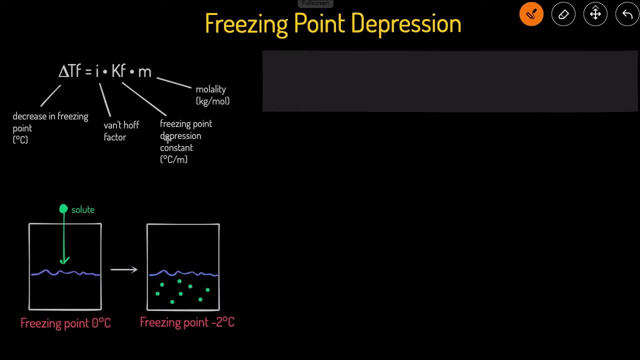 Times, the KF, which is the freezing point, depression constant- And this is a constant that's unique for every solvent- And the units for that change. it's in degrees Celsius divided by molality, And then the final variable is lowercase m molality, which is equals to kilograms. 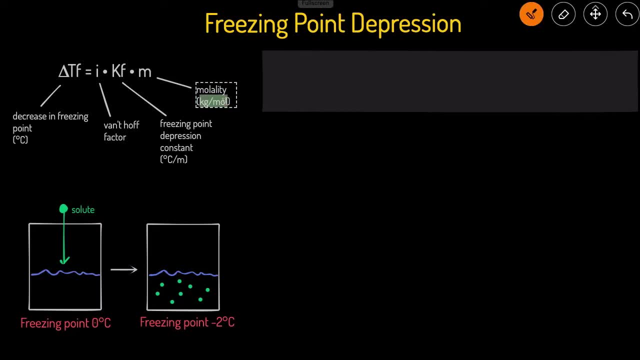 of solute divided by whoops. Actually, let me switch that. Actually it equals the most of the solute divided by the kilograms of desolvent. Great, Now let's take a look at an example problems of how we can use this equation. 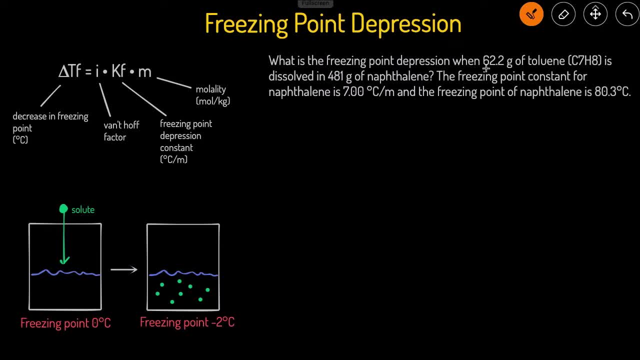 So this problem is asking us what's the freezing point depression when 62.2 grams of Tulene is dissolved in 481 grams of naphthalene And this gives us the freezing point depression constant, as well as the freezing point of the naphthalene before we dissolve the Tulene. So right off the 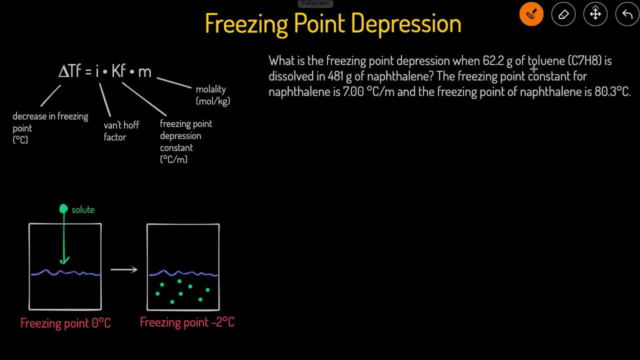 bed. we're expecting that, after dissolving the Tulene, the new freezing point will be lower than the original freezing point of 80.3 degrees Celsius. Since this question is asking about us, about freezing point depression, let's start with the freezing point depression constant And let's take a look at what 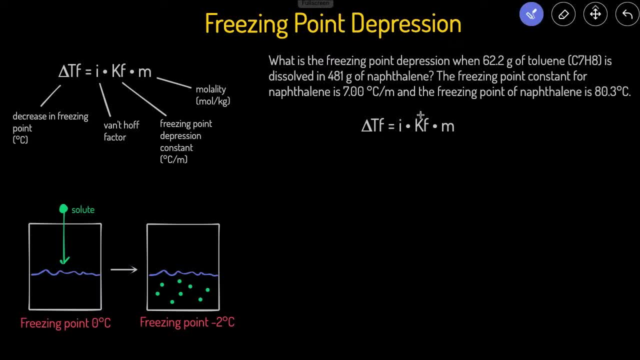 variables are already given to us. We already know the freezing point depression. We already know the freezing point depression, constant KF. Uh, we also already know. I first of all Tulene is. this is the solute, This was, that's what we're dissolving. 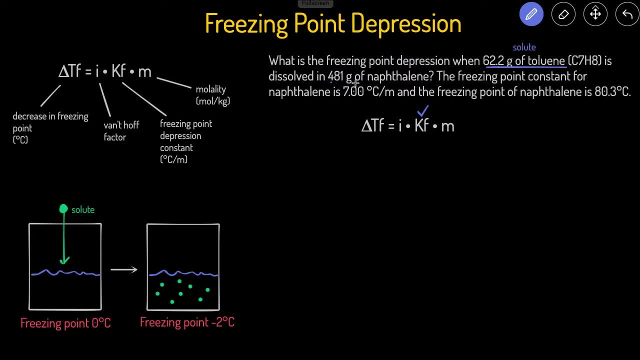 And then the naphthalene. This is our solvent. That's what's doing dissolving Tulene. It's the formula shown right here: C7H8.. We know this is a molecular substance because it just contains two nonmetals. And again, molecular substances do not break up into ions or separate when you. 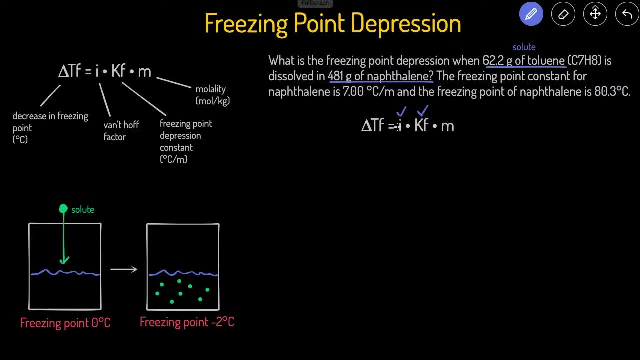 dissolve. So that means that we know that the I value is one. So we have to I value, We have to KF, We got to solve for the molarity and our goal is to, in the end, get to the change in the freezing point. 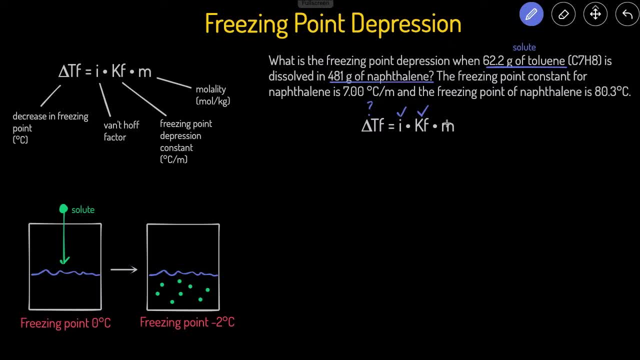 So let's start by solving for- sorry, I said I mean molality, where you got. We have to first start by solving for the molality. So molality is equal to the moles of the solute divided by the kilograms of the solvent. 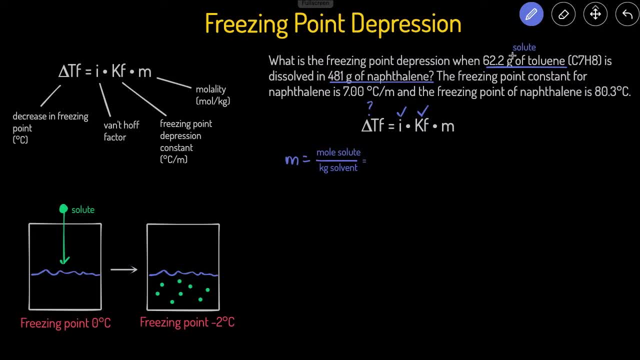 So let's get the moles of the solute. The way we get to the moles is we have to take the sixty two point two grams of the Tulene. The way we get to the moles is we have to take the sixty two point two grams of Tulene. 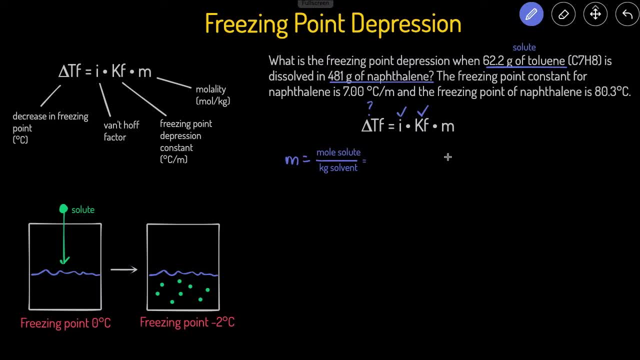 then we have to divide it by its, its molar mass. so we do 62.2 grams of c7h8 and then we have to divide by its molar mass, or we can write it as multiplied by one mole of the c7h8 divided by its. 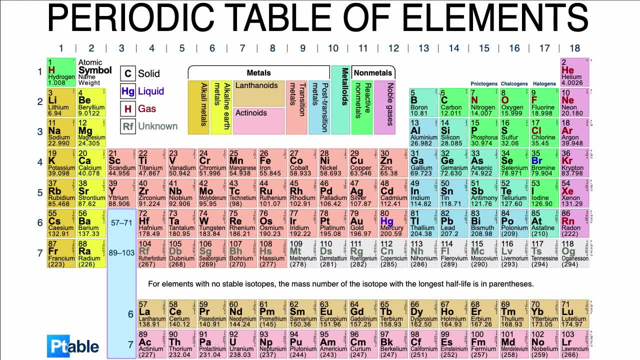 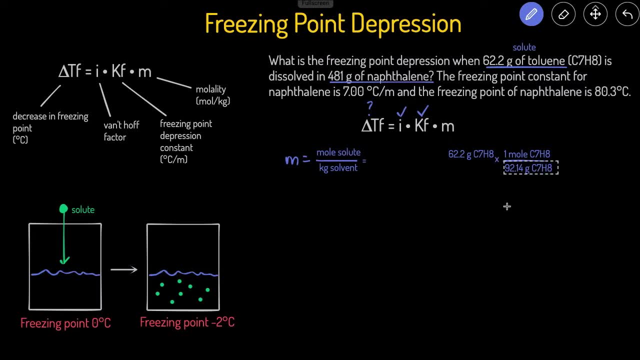 molar mass. and the way we get to the molar mass is just to add: take the molar mass of carbon multiplied by seven times the molar mass of hydrogen and multiplied by eight, and then, when we do that, we get a molar mass 92.14 grams of c7h8 for every one mole. so we take 62.2 divided by 92.14, that's 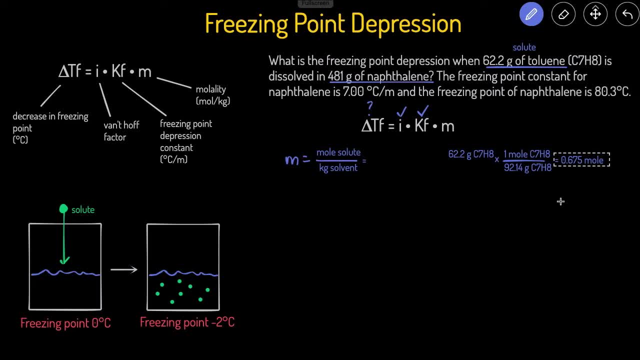 0.675 moles. so we got the top portion, 0, 675 moles. and then we have to divide by the kilograms. oh, we have the grams 481. so you get the kilograms. you just take the grams and divide it by a thousand and then that will give us 0.481. 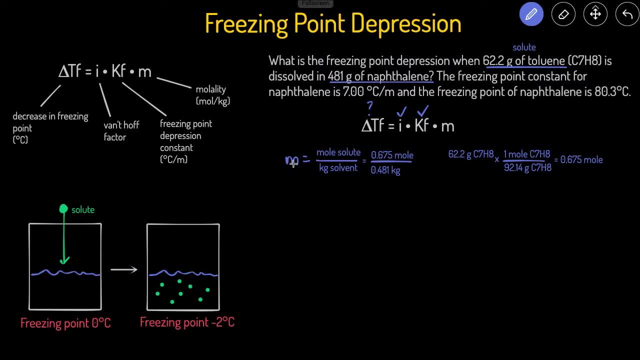 kilogram. now we take the top number divided by the bottom number and that'll give us the molality which is lowercase m right here, which is equal to 1.40 molal. now that we have the van hof factor, we have to kf. when we have to molal, let's plug it into the equation to get the change in the freezing. 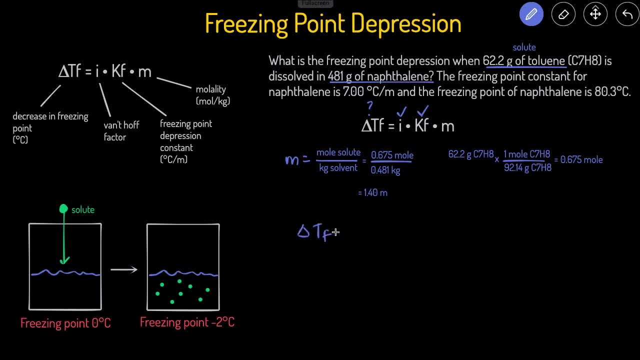 point. so the change in the freezing point is equal to the van hof factor, which we said was one, because then this is a molecular substance that does not dissociate- times the kf seven point zero zero degrees celsius, divided by lowercase m, times the molal that we got previously: 1.40. 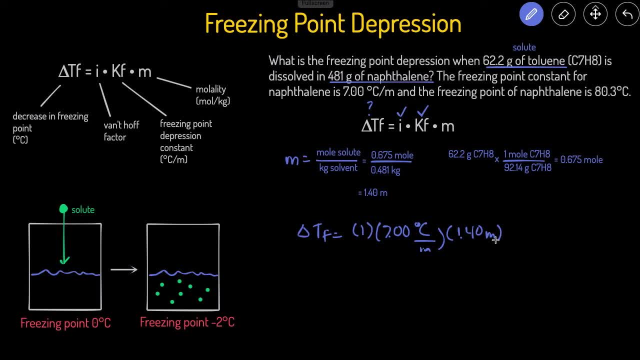 molal. plug that in and that gives you 9.82 degrees celsius. so that means the new freezing point will be 9.82 degrees lower than the original freezing point. all this question was asking us is: what's the freezing point? depression. so our answer: could, we can just say it's 9.82. but if we wanted to figure, 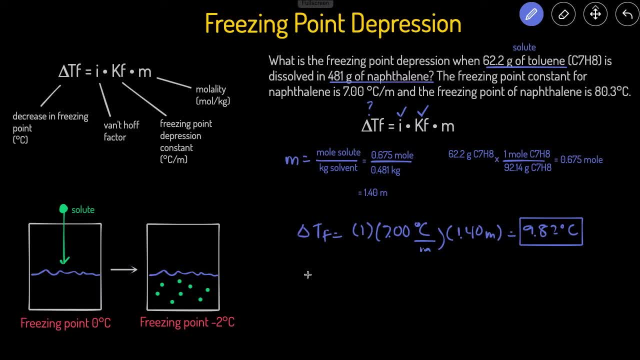 out the new freezing point the way we do, that is, we take the original freezing point of 80.3 degrees celsius and then we subtract the change 9.82, and so that means that the new freezing point is going to be 7.70.5 degrees celsius. after dissolving the toluene in the napoleon great. 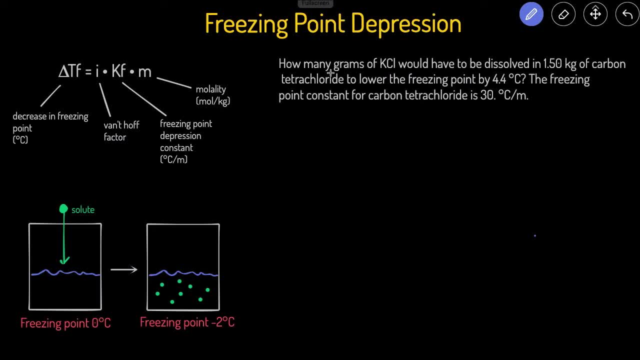 now let's take a look at a second problem. this problem asks us how many grams of potassium chloride, kcl, to be dissolved in 1.5 kilograms of carbon tetrachloride to lower the freezing point by 4.4 degrees celsius. so once again we're talking about freezing point depression. let's start with. 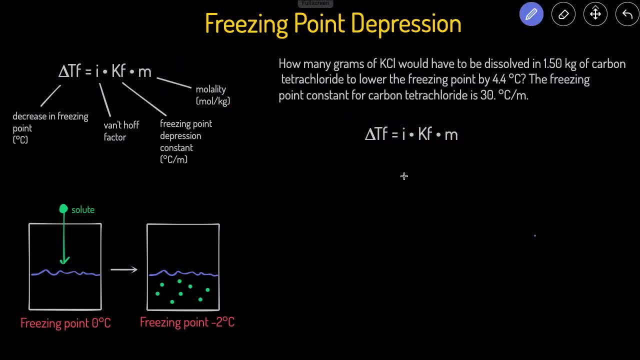 just the equation and take a look at what we are, what we already have and what we're trying to solve for. so we already have the change in the freezing point. it tells us that the freezing point is being decreased by 4.4 degrees celsius. so we already have that. we can figure out the i. 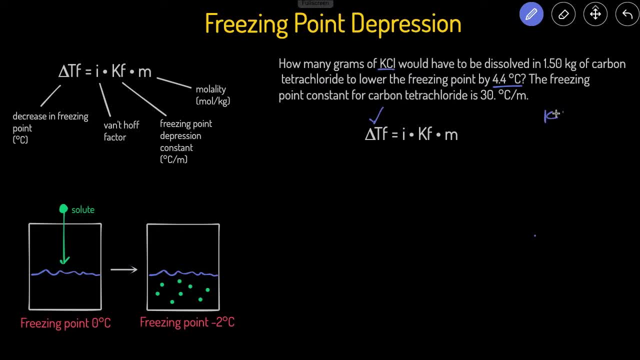 we know that kco is an ionic substance. so that's going to break up into k plus the cation and then co minus the anion. so you can see, it breaks up into two substance, two ions. so that means that the i value is going to be two. so we have this as well. it tells us the freezing point constant. 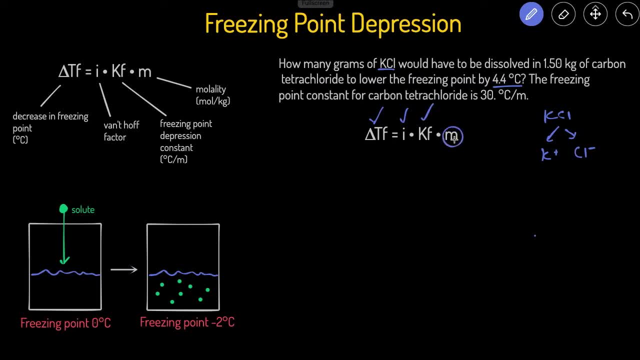 right here, so we also have that. so then we should probably start by solving for the molality, and then from there we can get to the grams of the kco. the change in the freezing point is going to be 2.5 degrees celsius, so we already have that. so we already have that. 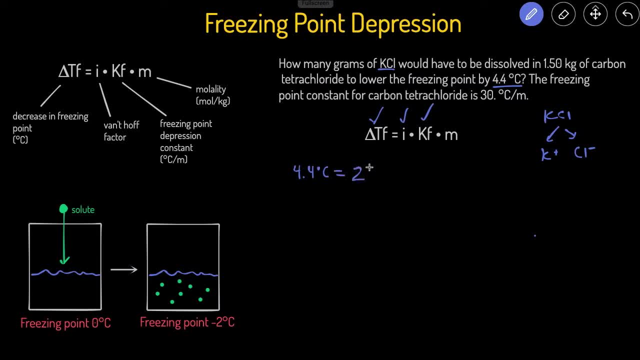 point is 4.4 degrees celsius. we said that the i value is 2, the kf is 30 degrees celsius per molal, and then we're solving for m. so to do this, we just we just take the 4.4 degrees celsius and 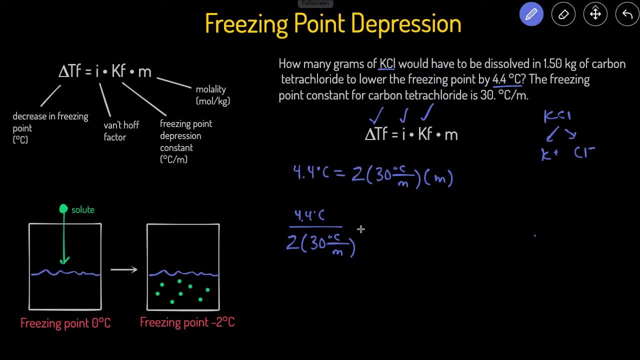 then divide it by 2 times 30 and that'll give us the capital m, which is equal to 0.0733. and remember, capital m is equal to the moles of the solute divided by the kilograms. so let's rewrite that right here: this is going to equal the moles of the solute and our solute was the kco divided. 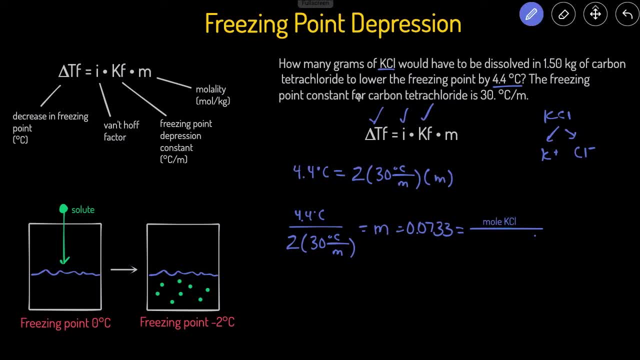 by the kilograms of the solvent, which is the carbon tetrachloride. and we already have the kilogram, so let's plug that in. so our next step: we can just cross, multiply it. we can multiply 1.5 by the point zero. seven, three, three, and that'll give us the moles of the kco. so the moles of kco. 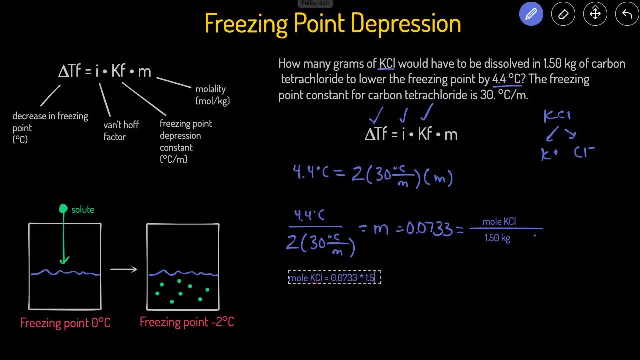 equals 0.0733 multiplied by 1.5 and that's 0.11 moles of kco. now that we have the moles to get to the grams, we just have to multiply by the molar mass. so we'll set it up: 0.11 moles of kco multiplied by. we want to put 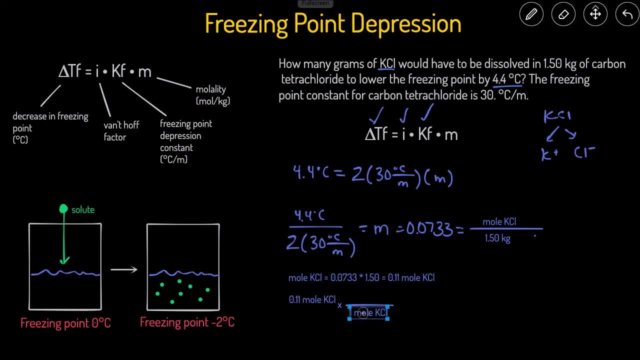 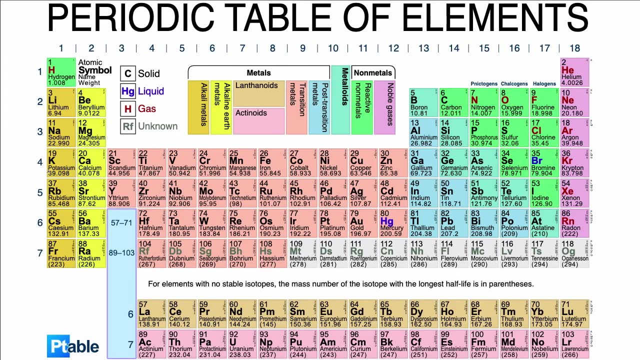 the one mole of kco on the bottom. so it can cancel out. remember molar mass is how many grams there are in one mole and then to get the molar mass we can go take a look at k molar mass plus cl's molar mass and then that's 74.55 grams of kco. 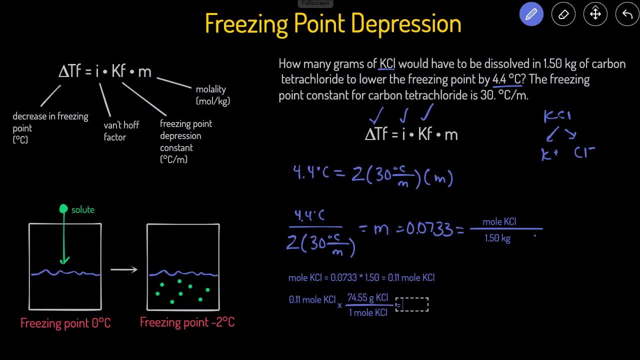 so 0.11 times 74.55 gives you 8.20 grams of kco as the final answer. and there you have two examples of freezing point depression. just when you read the problem, and it mentions freezing point depression. start by writing this equation out and then think about which variables are. 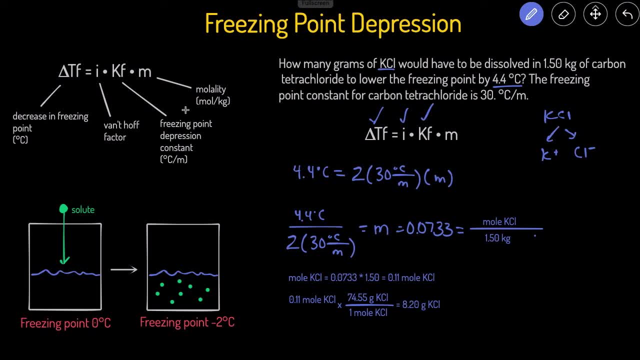 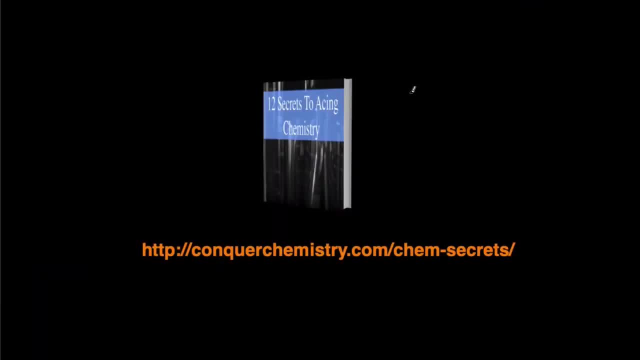 you already given and which ones you are solving for. if you want to learn how to ace chemistry. if you want to learn what's the best way to study for this class. if you want to learn some neat tricks and tips to take into your exam and do better on. 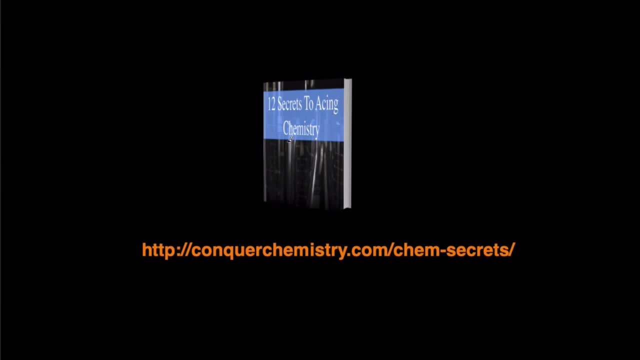 them, then you should head over to my website and get this free guide: 12 secrets to ace in chemistry. you can head over to wwwconquerchemistrycom. slash chem secrets. i'm going to include a link in the description below. check it out. i think it's really going to help you. 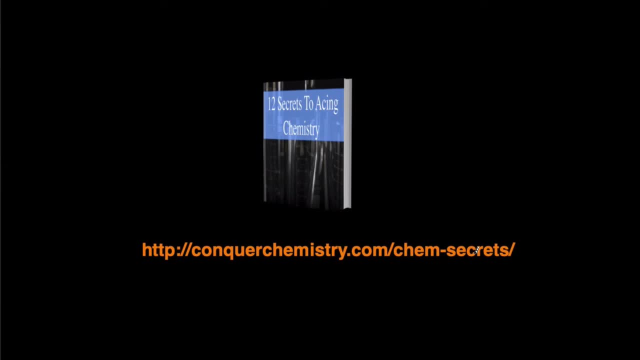 and you're going to- you're going to like it- until next time. keep working hard and continue the good work.